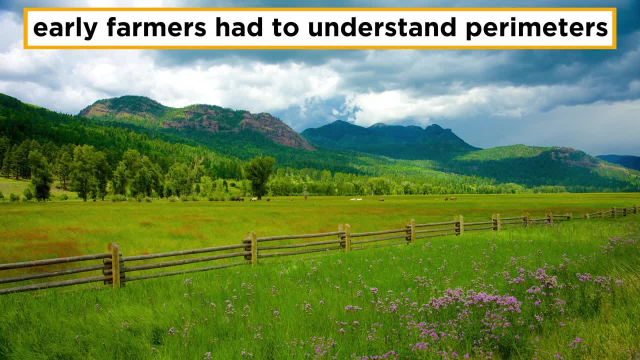 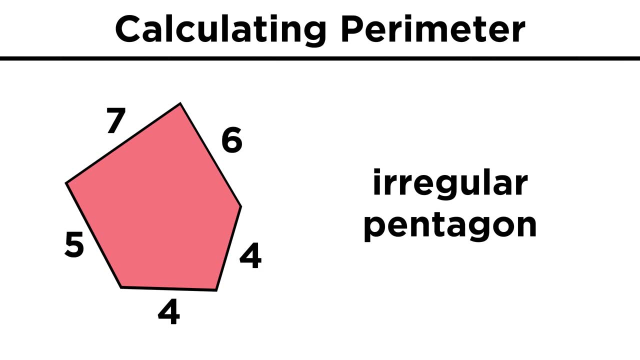 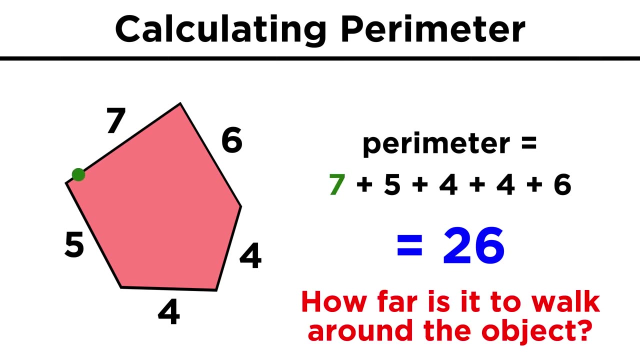 how much material they needed to enclose their land and guard their animals or crops. Here is an irregular pentagon. Given these side lengths, we just add them up And that's the perimeter. This is the same thing as asking if you walked along each edge of the shape all the way. 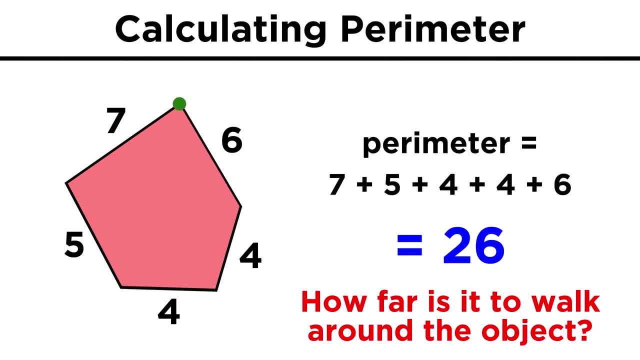 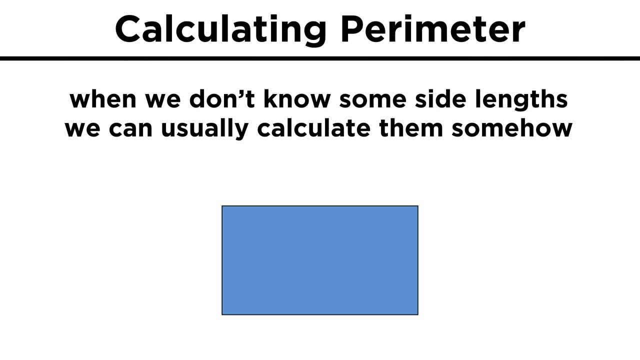 back to where you started. how far did you walk? If we don't know one or more of the sides, we can usually calculate them depending on what shape we are looking at. First, let's look at rectangles. These have both a length and a width. 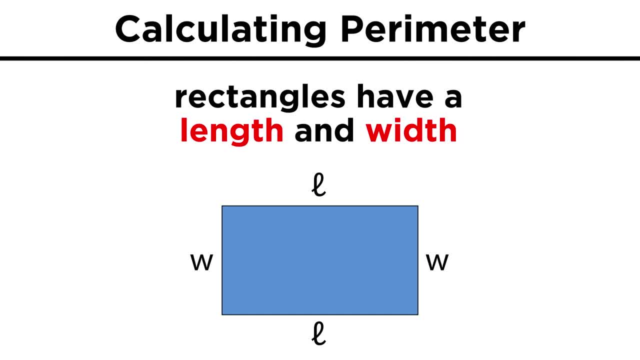 Since there are four sides, total two lengths and two widths, The perimeter of a rectangle is equal to L plus W plus L plus W, or two L plus two W. So if the dimensions of a rectangle are four by two, we can just plug these into the equation. 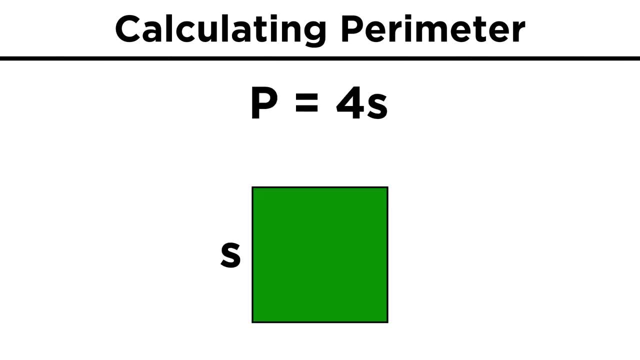 and we see that we get twelve for the perimeter. For squares it's even simpler: it's just the side length times four, since all the sides are the same. Sometimes we may be given a perimeter problem that we can do algebra with. 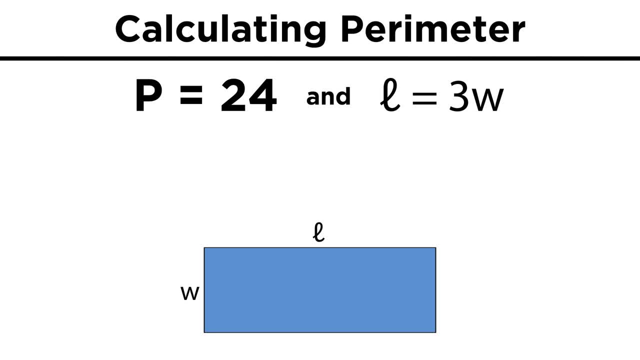 Say we have a rectangle. Let's say we have a rectangle with a perimeter of twenty-four and its length is three times its width. What are the dimensions of the rectangle? Well, we know that two L plus two W must equal twenty-four. 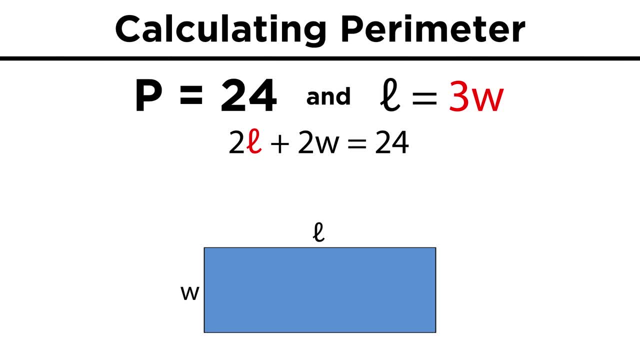 We also know that L equals three W. Remember how to solve two equations with two unknowns by substitution. Let's put three W in place of L in this equation, which gives us six W plus two W, or eight W equals twenty-four. 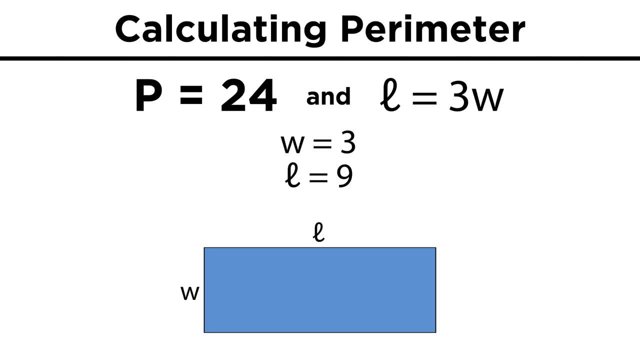 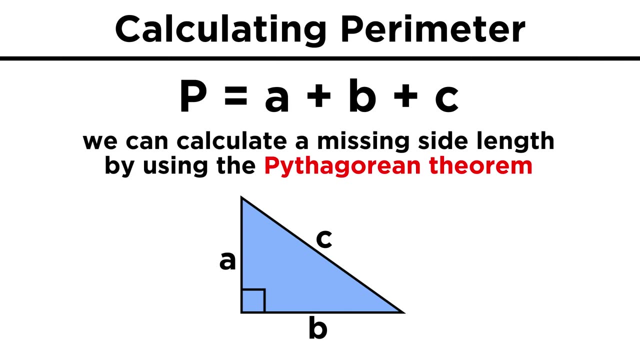 We divide by eight, W must be three and therefore L must be nine. The rectangle is three by nine. If we have a triangle, again we add up the sides, and if we have a right triangle with an unknown length, we know that we can use the Pythagorean theorem to find the missing. 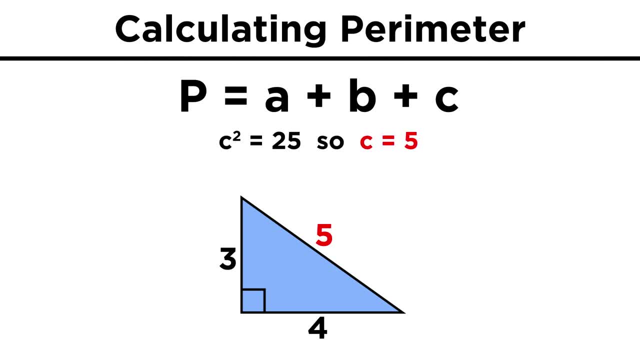 side Like this one. if the legs are three and four, we know the hypotenuse must be five and the perimeter is therefore twelve. Sometimes we may be given a problem that we don't know how to solve. We divide by eight, W must be three and therefore L must be nine.